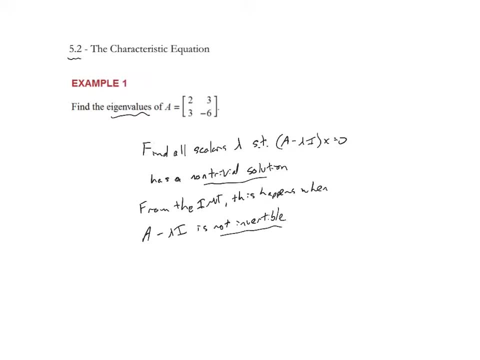 And what's the easiest way to find out? if my matrix is not invertible, We can find its determinant. So we find the determinant of A minus lambda times the identity. Alright, that's the big key here. That determinant is going to give us our eigenvalues. 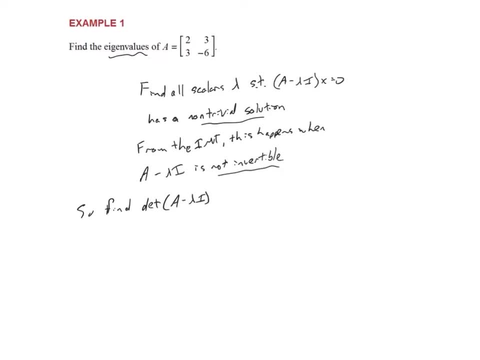 So in terms of the work here, the first thing that we're going to do is find A minus lambda times I, So A minus lambda I is equal, to remember. we just subtract lambda on the main diagonal: 2 minus lambda, and then 3 here, 3 here and negative 6 minus lambda right there. 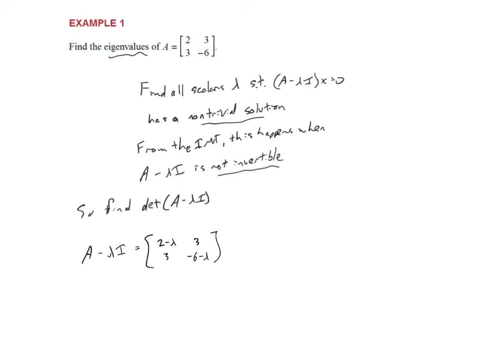 And then the determinant of this matrix, A D minus B C. we have that formula: The determinant of A minus lambda I is equal to okay. so I'm going to write this out. We're going to multiply 2 minus lambda times negative, 6 minus lambda, and then subtract 9, so minus 3 times 3.. 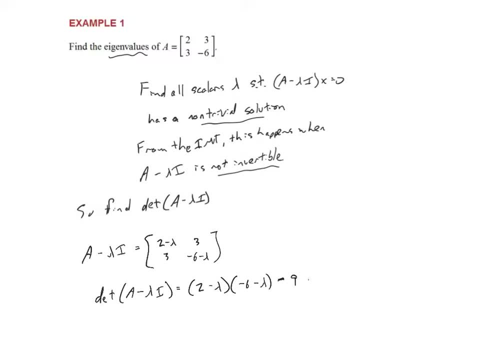 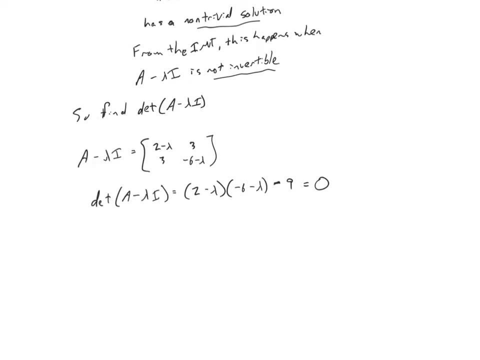 Alright, there's our determinant. When you and we're going to set that equal to 0- because I want to find when that's 0, then my matrix is not invertible. When you distribute and simplify, you get lambda squared. 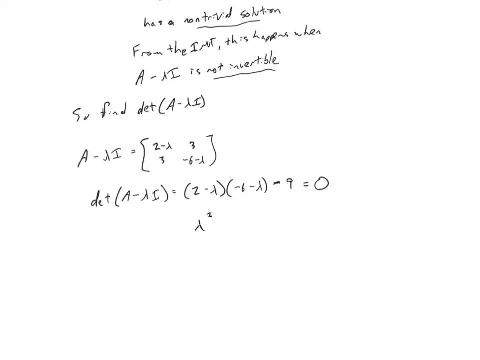 Oops, that looks terrible. Try that again. Lambda squared then plus 4. lambda minus 21 equals 0. So we're doing a little regular algebra in the middle of this problem. We distribute, simplify factor: Lambda minus. 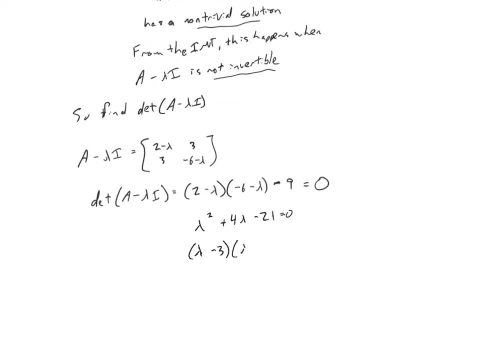 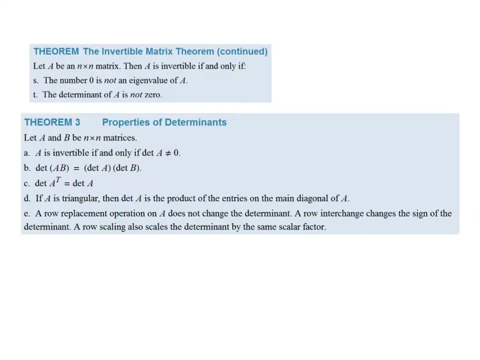 Minus 3 times lambda plus 7 equals 0. So that tells me that lambda equals 3 or lambda equals negative 7. And we have our two eigenvalues for this matrix. We get a couple of theorems on this next slide here. 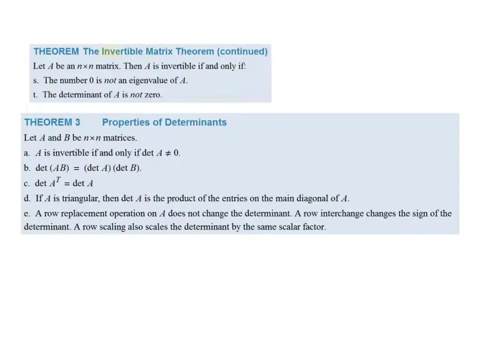 The first one being: well, hey, the invertible matrix theorem. That should look familiar, but now we add on two more letters. We're already up to S and T in the alphabet. So for a matrix, being invertible is now equivalent to the number 0 is not an eigenvalue of A. 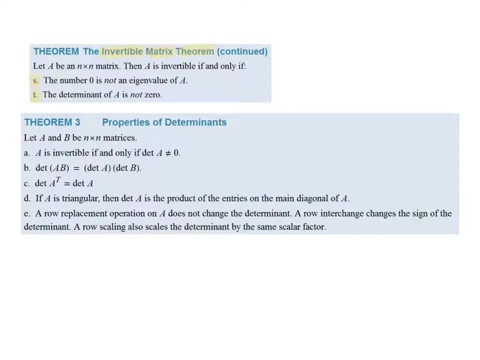 And the determinant of A is not 0. We've known that for a while Now. it's officially formally included in the invertible matrix theorem. But we also get this clause about the statement about the eigenvalue, And then theorem 3 on the slide: properties of determinants. 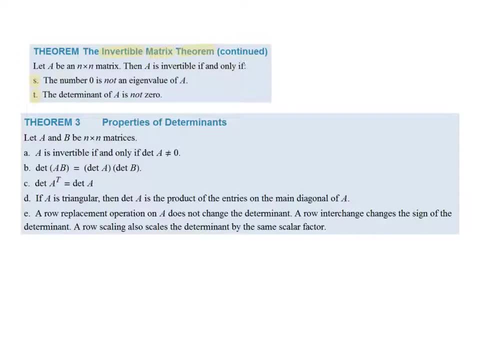 This is essentially review. We've seen these properties before. So A is invertible If, and only if, the determinant is non-zero. The determinant of a product is a product of determinants. The determinant of the transpose of a matrix is the determinant of its original. 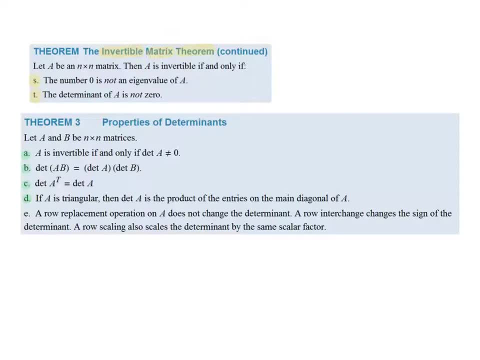 If A is triangular determinants of the products along the diagonal And then row replacement operations do not change the determinant. Okay, so those are. we've seen that theorem before. It's being brought back here in this section, just to kind of refresh your memories. 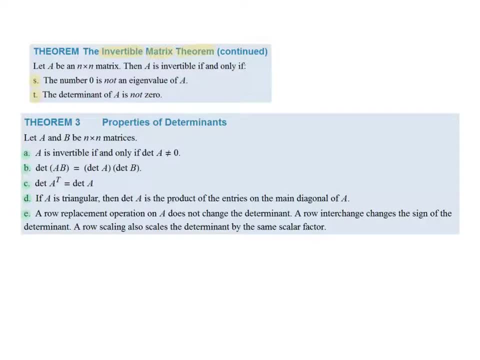 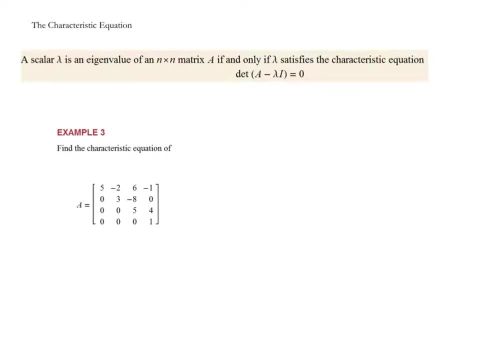 There's another example that I'm leaving off to just remind you about Determinants, because we've been away from them for a chapter or so. Okay, now we get to the main topic in this section, And that is the characteristic equation. 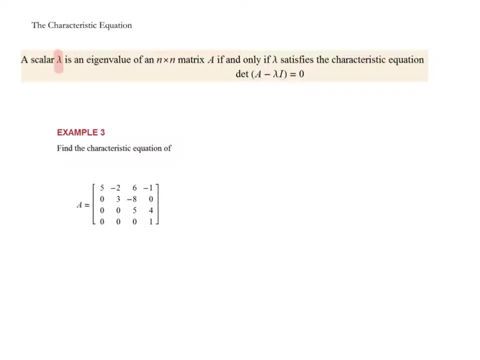 So a scalar lambda is an eigenvalue of a matrix, n by n matrix, If, and only if, it satisfies the characteristic equation of this. The determinant of A minus lambda I equals 0. So that's what is called. when you compute that determinant, that equation is called the characteristic equation. 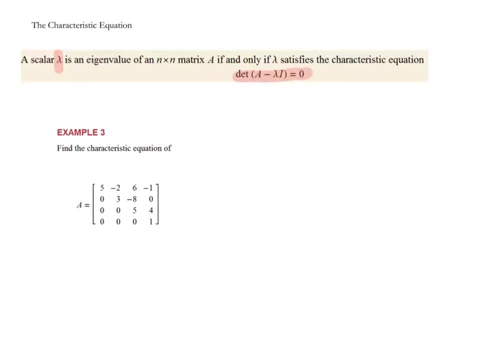 And then in example 3, we're going to find a characteristic equation of a triangular matrix, Because that's a little bit easier to work with. So for our matrix A, we're going to write down first A minus lambda times the identity. 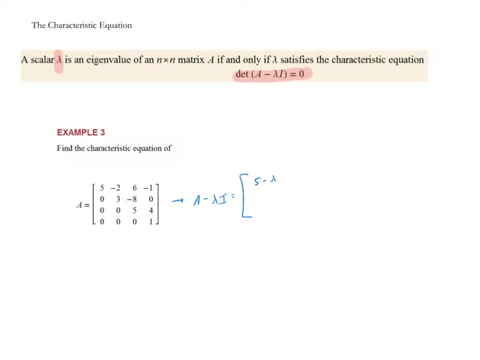 And that is equal to 5 minus lambda up top with a couple of zeros or three zeros below it: Negative 2.. 3 minus lambda. with two zeros: 6,, 8, negative 8.. 5 minus lambda. 5 minus lambda. 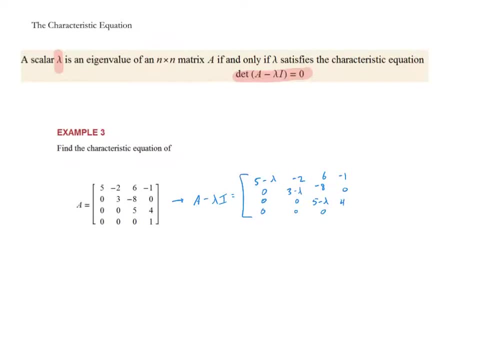 5 minus lambda, with a single zero Negative, 1,, 0,, 4, and 1 minus lambda at the bottom. Okay, and so the reason in this example, this first one, where we're introduced to the characteristic equation that we have a triangular matrix, is because in that theorem that we just had our memories refreshed about, 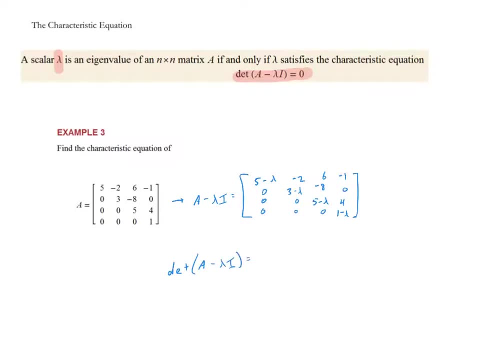 the determinant of A minus lambda times. the identity is just the product of the entries along the main diagonal: 5 minus lambda, 3 minus lambda, 5 minus lambda And 1 minus lambda. Oh, that's a terrible lambda, but we'll go with it. 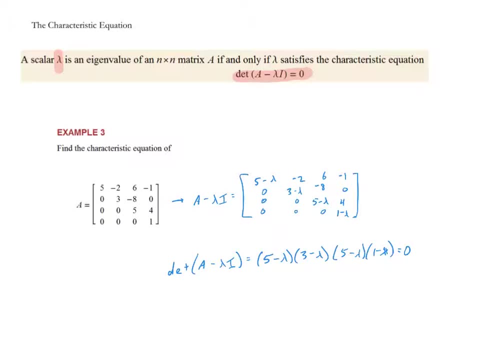 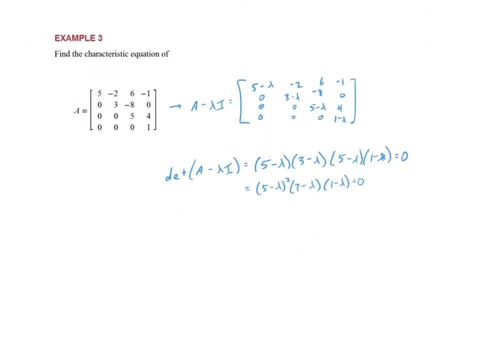 Equals 0.. So there is my characteristic equation, okay, And so we could even simplify this a little bit: to 5 minus lambda squared, 3 minus lambda, 1 minus lambda equals 0.. Okay, so there's our characteristic equation. 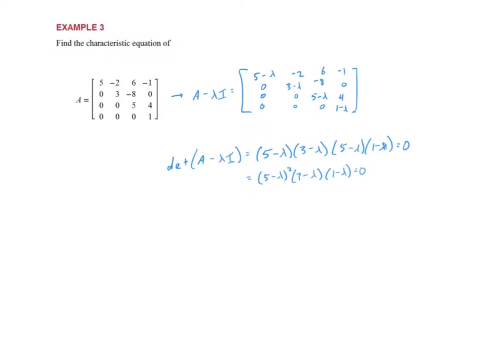 And then let's just say a couple of things here. We can see what our eigenvalues are. We are at this point, I hope. But the eigenvalue 5 has what is called a multiplicity of 2.. And you may have heard of 2.. 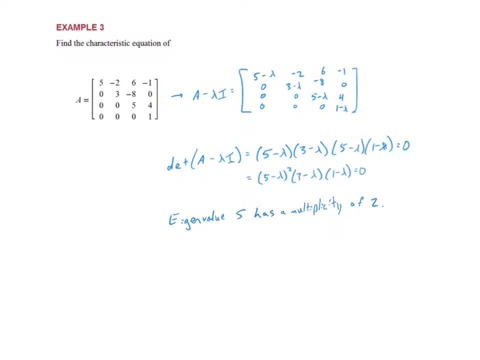 And you may have heard of multiplicity in the past in dealing with graphing polynomials. It has to do with how it intersects the x-axis, whether it passes through or just skims off of and goes back up. But that's the degree of the exponent there. 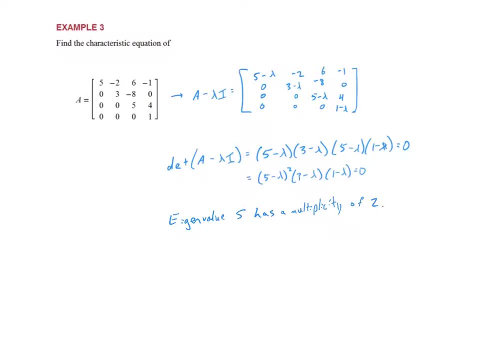 It means that the multiplicity is 2.. And then let's see what else did. I want to say So because lambda minus 5 appears twice in the character, or 5 minus lambda appears twice in the characteristic equation. 3 and 1 would both have a multiplicity of 1.. 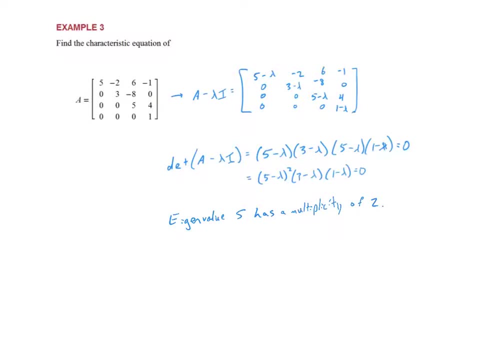 Something else that I will just define by example. here We have what is called the characteristic characteristic. there we go polynomial. Okay, If I take all of those factors and multiply them out, I get lambda to the fourth minus 14 lambda cubed plus 68 lambda squared minus 130 lambda plus 75 equals 0.. 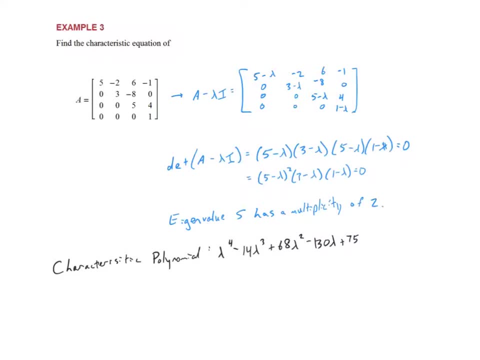 But if I drop off the equals 0, then that is called the characteristic polynomial for my matrix A And that you factor to find Your eigenvalues. Okay, For this next example, we're given a characteristic polynomial for a 6 by 6 matrix. 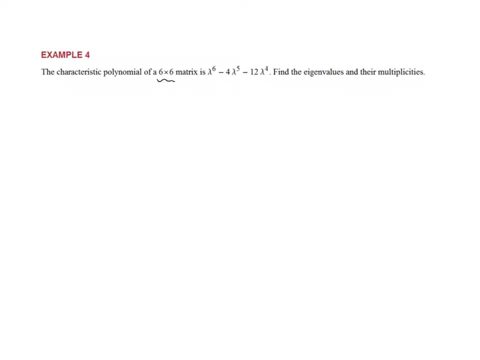 Luckily we didn't have to do this one, this determinant, by hand, But what I can do to find its eigenvalues is factor And if you factor- and, by the way, your calculators, if you didn't already know, they have a factor command. 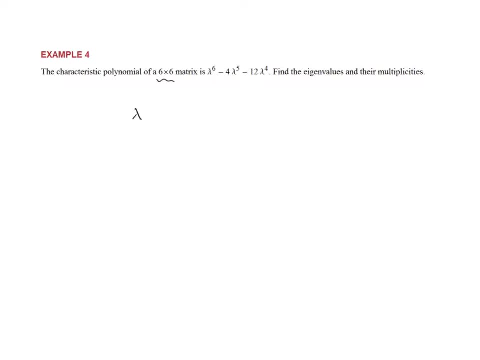 So from the home screen, if you hit let's see what is it? F2, number 2 is the option to factor, And then you just type that polynomial in And it will factor it for you. Spit it out in its factored form. 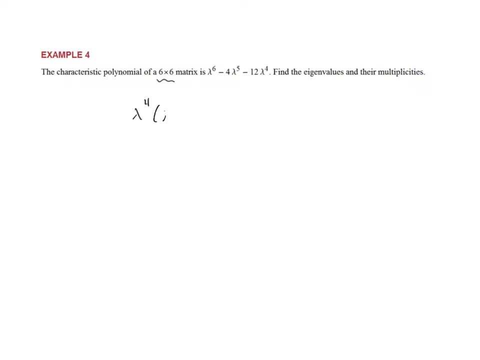 But if you do that here, you get lambda to the fourth times lambda minus 6 times lambda plus 2.. Okay, So that is my characteristic polynomial. And then lambda equals 4, or lambda equals 0, rather, Lambda equals 0 has multiplicity. 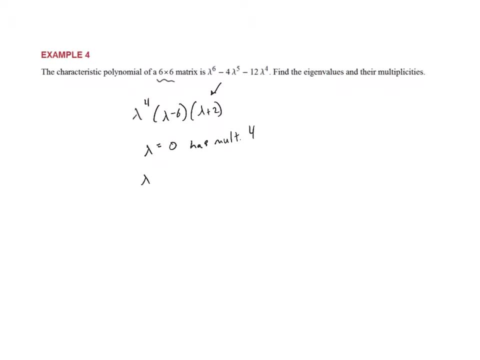 I'm going to abbreviate that: 4.. Lambda equals 6 has multiplicity, Multiplicity 1.. And lambda equals 2 also has multiplicity 1.. There we go, Okay, So that is all we had to do for that one. 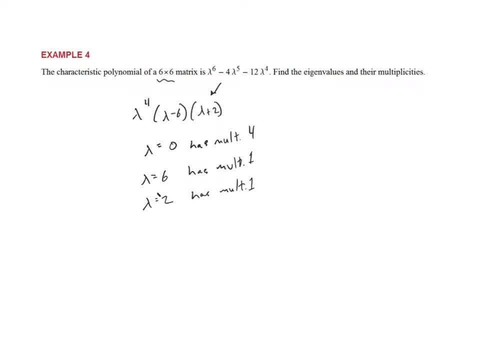 Oh, that should be. lambda equals negative 2. Whoops, There we go, Squeak that in there. Okay, Now we're going to transition to talking about something called similarity. So I'll define that first, And then I will see how that ties in in the theorem right below. 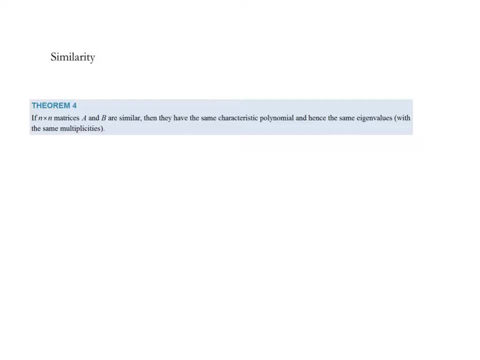 Ties into eigenvalues. Okay, So similarity: A is similar, A is similar to B, So two matrices are similar. If there exists, If there exists, EX Whoops, If there exists- an invertible matrix P Such that 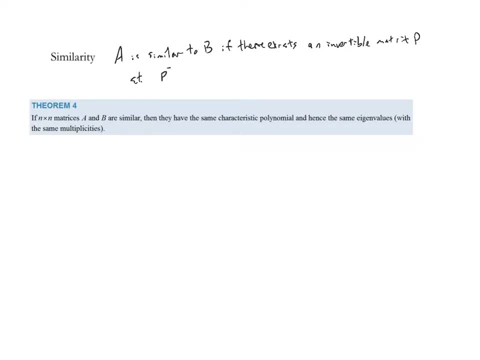 S-T, for such that P inverse times A times P is equal to B Or, equivalently, A equals P, B, P inverse. Okay, So that is what it means for two matrices to be similar. They're basically the same if I multiply one of them by a matrix. 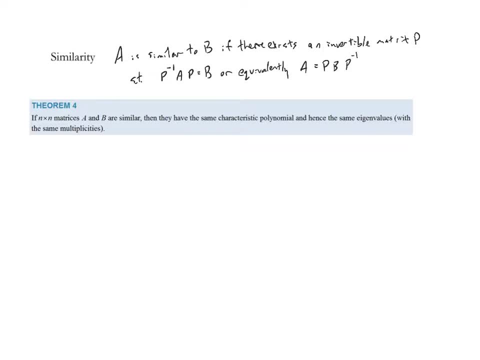 Okay, by a matrix, another matrix and its inverse. so that's kind of a cool relationship that exists with. matrices a and b are not the same, but they're pretty close because when i multiply them by this other matrix they are the same. multiply one of them by this other matrix and its inverse, they 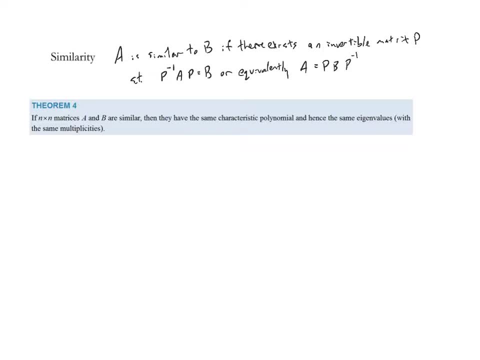 are the same. okay, so that's our definition for similar. and how does that tie into eigenvalues? why is that important here? well, the theorem says: if two matrices, a and b, are similar, which we've just defined- then they have the same characteristic: polynomial. if our goal is to find more eigenvalues, 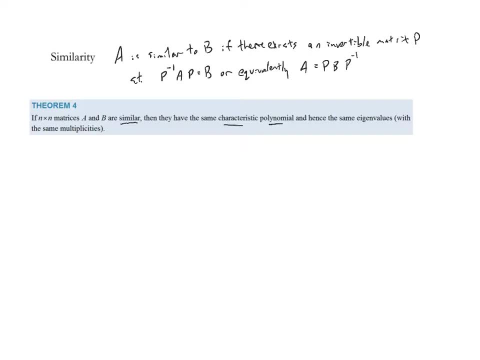 well of matrices. here we have a way to make the to maybe make the process more efficient. two matrices are similar. they have the same characteristic- polynomial- and hence the same eigenvalues with the same multiplicities. so that's pretty cool. similar matrices have the same eigenvalues with the same multiplicities- all right, and i want to go through a proof of this one. 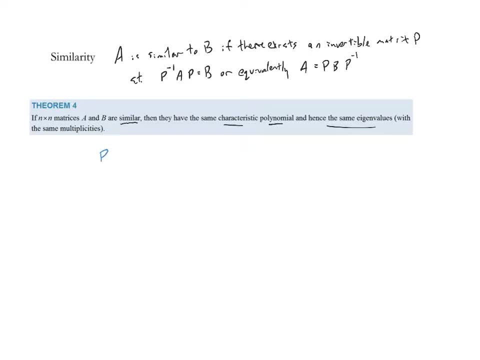 because it's kind of interesting, i think. so let's take a look at it. proof: all right, if if b equals p inverse times a times p, because they are similar, then b minus lambda times the identity is equal to p inverse a, p minus lambda times p inverse p. so let's take a look at what i did there. 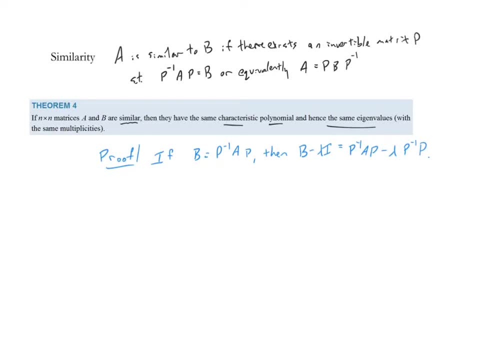 so i just wrote it down. but let's see what i actually did on the left hand side. let me get my highlighter. there we go. i subtracted lambda times the identity. so from the left hand side, i subtracted lambda times the identity. on the right hand side, i subtracted- take a look at that. 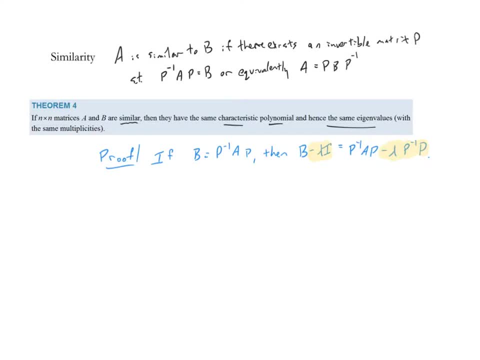 lambda times the identity. so i basically wrote the same equation on the left but subtracted lambda times the identity on both sides. i just wrote it in a particular way on the right hand side, and the reason that i wrote it that way is because i know where i'm going. 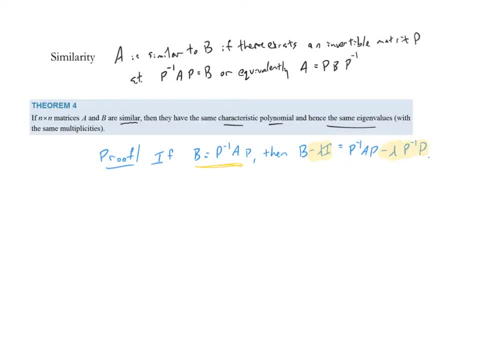 and ultimately i want to factor some things here. okay, so what can i factor? let me write this over here a little bit more so: b minus lambda times, the identity is equal to first. i'm going to factor a p inverse out on the left hand side: right, i have p inverse, right here i have p inverse. 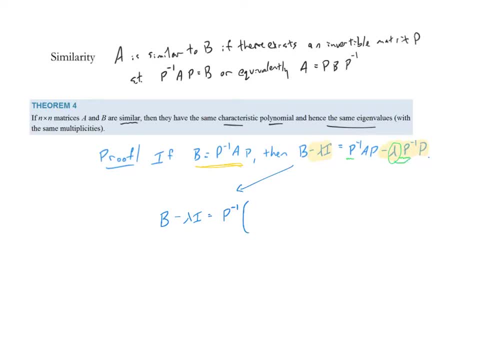 right here that lambda is just a scalar. so properties say that i could like multiply i could, i could change the order of the scalar and multiplication there so i can factor p inverse out and what's left in the first term ap minus in the second term. uh, lambda times p cool, so we factor. 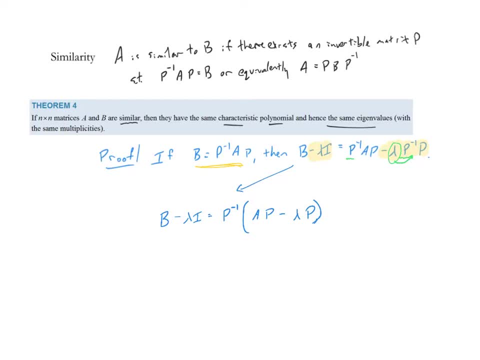 that out there. all right, maybe you can see where this is going in the next step. do you see the p's common to both terms? so i'll ask the question and then i'll answer it myself: where am i going to factor that p E? so where am i going to factor that p E? 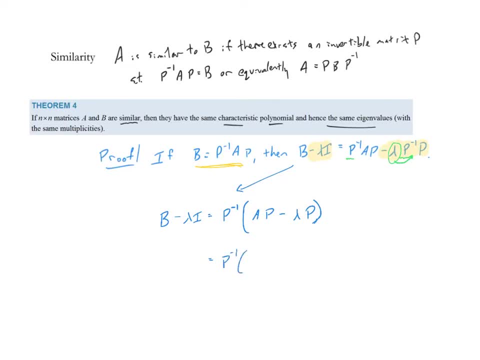 where am i going to factor that p, E, p out? i heard someone say on the right: uh, so inside of the parentheses i'm gonna have a minus lambda times the identity, and then we factor that p out on the right hand side. all right, so b minus. 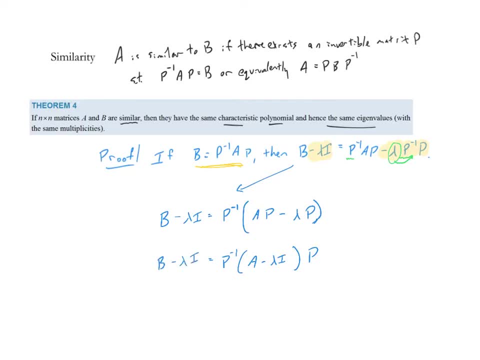 lambda i on the left hand side of the equation. p inverse a minus lambda i- p on the right hand side of the equation would be really, really great if i could get the p inverse and the p to be next to each other, because then i could just say that they're the identity and then cancel them out. 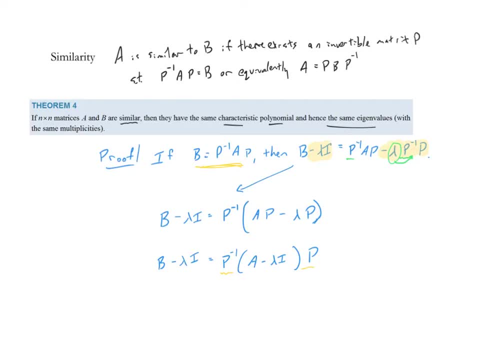 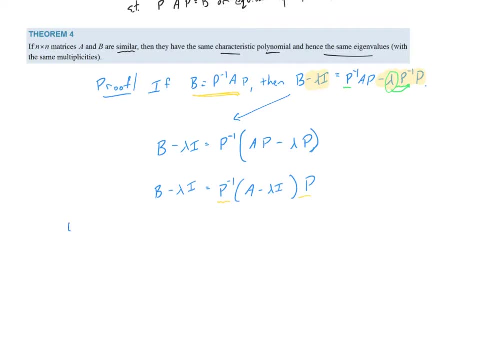 but i can't force that. that would be incorrect. all right, so what we do is using theorem three, and i'll write it down. that's the theorem that i showed a little bit earlier. using theorem three, we're going to take the determinant on both sides. we're going to take the determinant on the left. 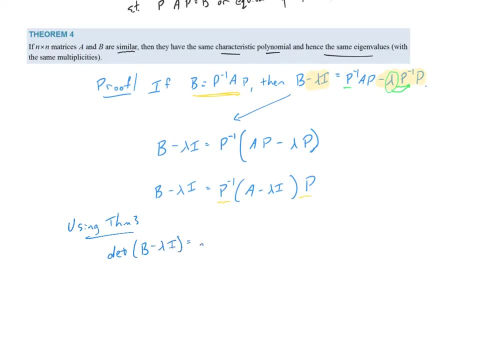 of b minus lambda times the identity and the determinant on the right of all that stuff- p inverse: a minus lambda i p. okay. the advantage of that is on the right product of a determinant of a product is the same as the product of the determinants- p inverse. 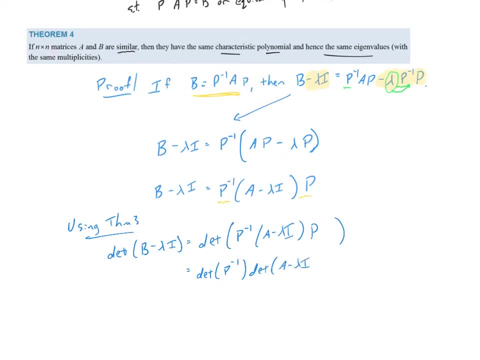 determinant of a minus lambda, i determinant of p. now remember, determinants are just numbers. the determinant of a matrix can be seven, so the determinants are just numbers. so can i commute numbers? the answer is resoundingly yes. so i could move things around now that i have 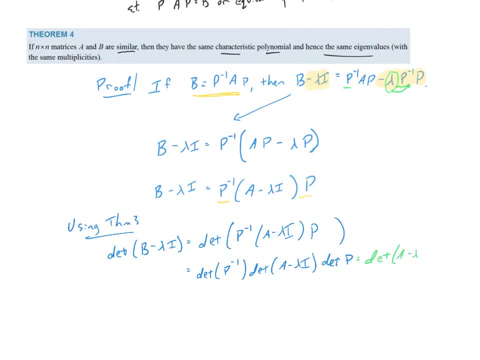 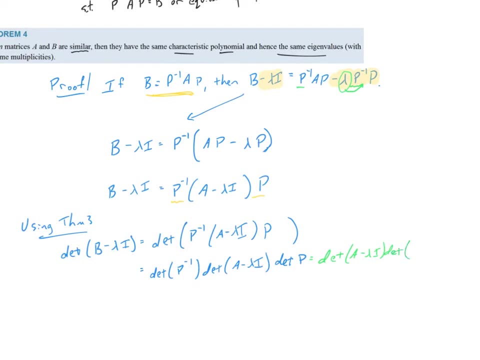 determinants. so the determinant of a minus lambda i is the determinant- let me move it over a little bit- here is the determinant of p, inverse times, the determinant of p which these two guys i can just put back together. so i'm kind of going all over the place with this problem. 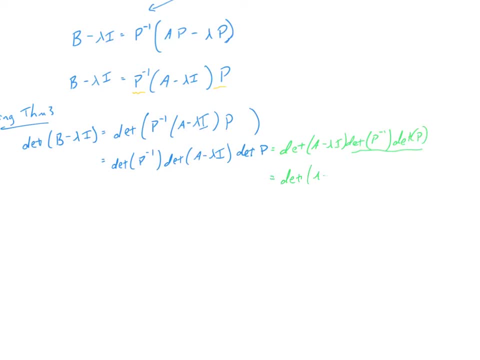 hopefully, that's all right. determinant a minus lambda. i times the determinant of p. inverse times p. oh man, this is awesome. and then that, well, p inverse times p. is this just the identity? the determinant of the identity is just one, and so all of that we're left with. 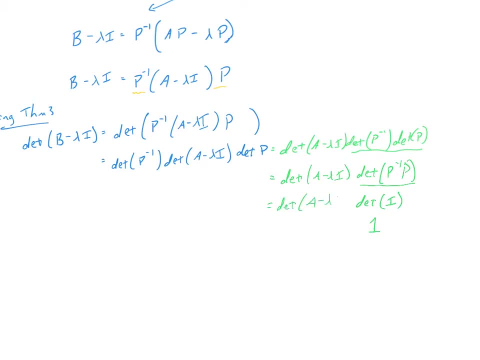 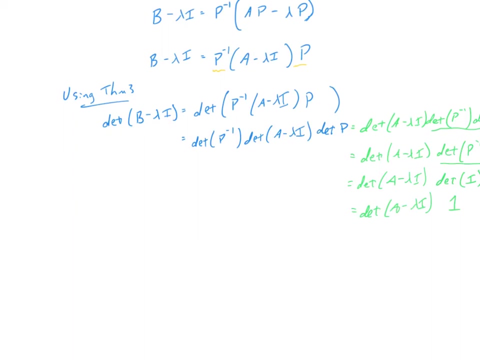 determinant a minus lambda. i let me just write it twice for consistency. determinant of a minus lambda. i right there, boom, um, and that's. that's basically the conclusion of the proof. let me write the two pieces next to each other, so it is kind of together. bring this. 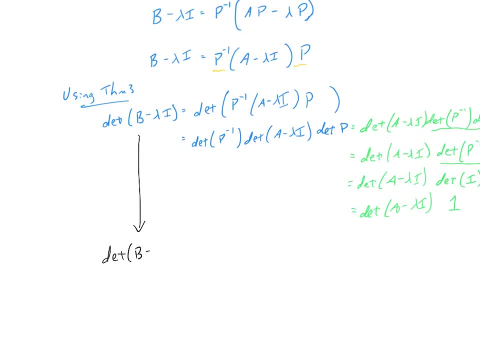 down, the determinant of b minus lambda i is equal to the determinant of a minus lambda i. and what does that mean? they have the same eigenvalues, they have the same characteristics, they have the same characteristics, they have the same characteristic equation, and that's pretty cool. so we've got this relationship between: 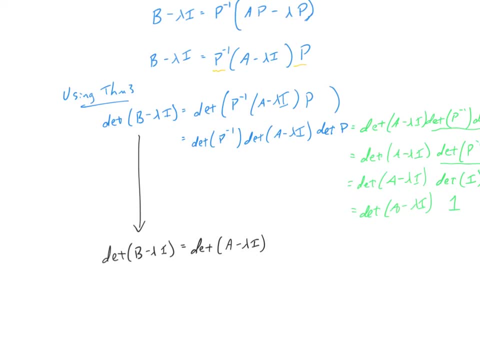 similar matrices and their eigenvalues. we'll close out the section with two uh little warnings here, and the first one: i'm going to write down two, oops, i'm going to write down two matrices, uh, this one here, two zero one two. and this guy here, two zero zero two. okay, so, those two matrices. 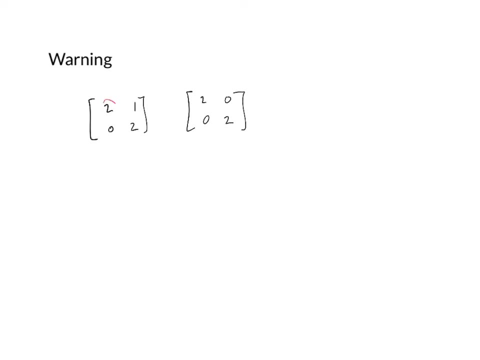 because they're triangular. i know their eigenvalues. they both have an eigenvalue of two and a multiplicity of two. however, these two matrices are not similar. so if they're similar, then they have the same eigenvalues. however, if they have the same eigenvalues, that does not mean that they are. 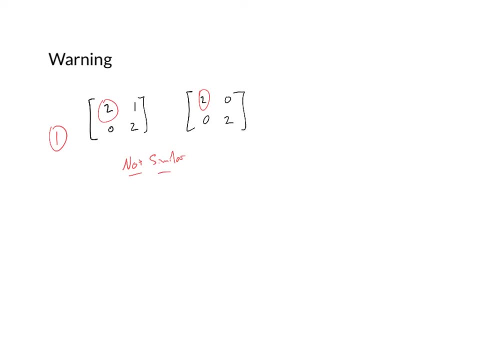 similar and that's warning number one. uh, warning number two: is similar, is similar, is similar, is not the same as row equivalent. okay, similar, row equivalent. those have two different meanings. so if you find the two matrices are similar and you use the tilde symbol, um, that is not correct. the tilde tilde, one of.